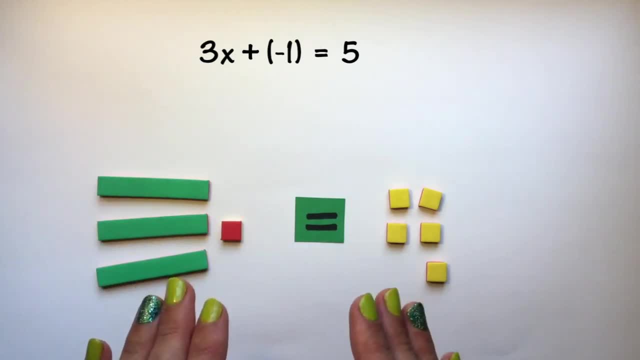 only variables on this side of my equation, no integers, So I'm going to need to remove negative 1.. I don't have a negative tile I can remove on this side, so I add a zero pair. Now that I have a zero pair, I can remove negative 1 from. 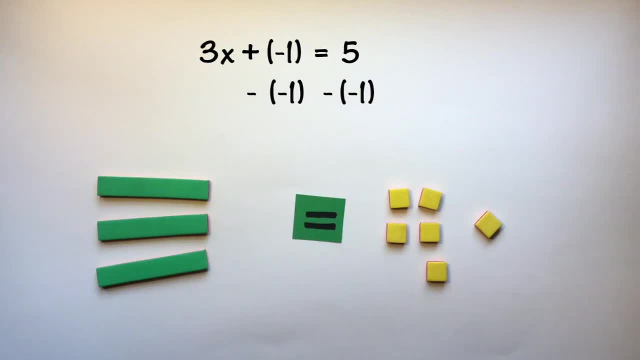 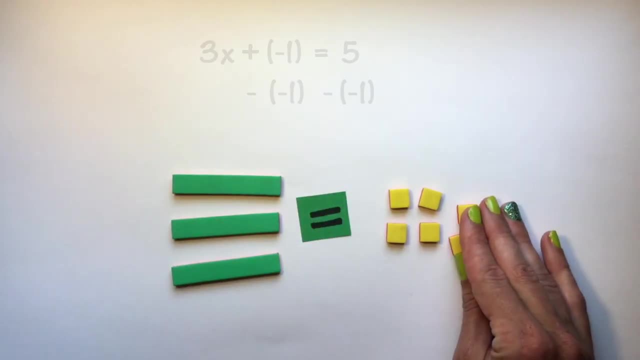 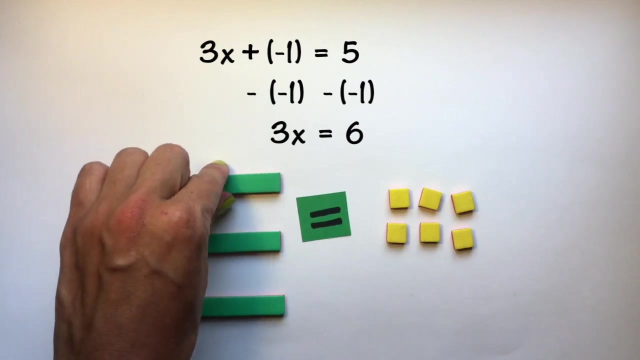 both sides of the equation, keeping it in balance. And now I have that 3x is equal to 6.. So to get one x by itself, I need to split my variables into three equal groups: One group of x, one group of x, one group of x. 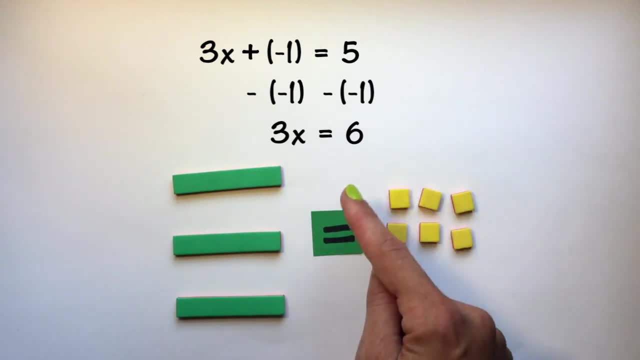 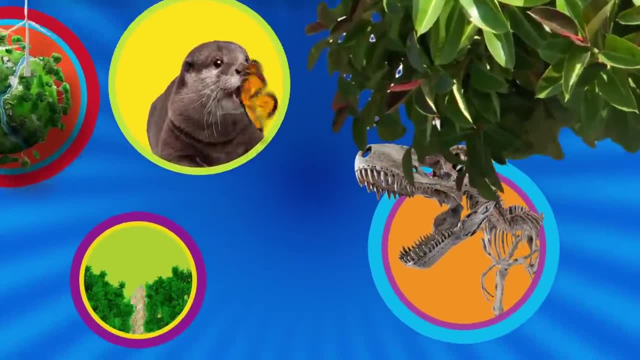 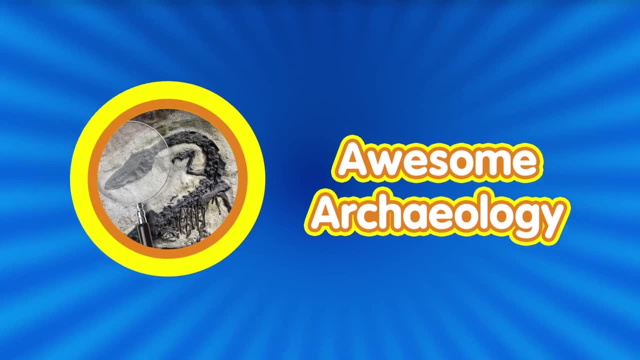 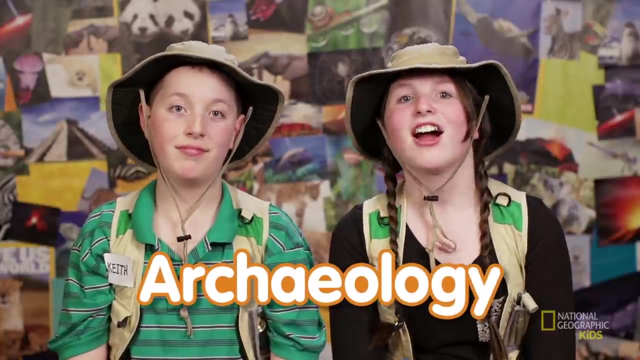 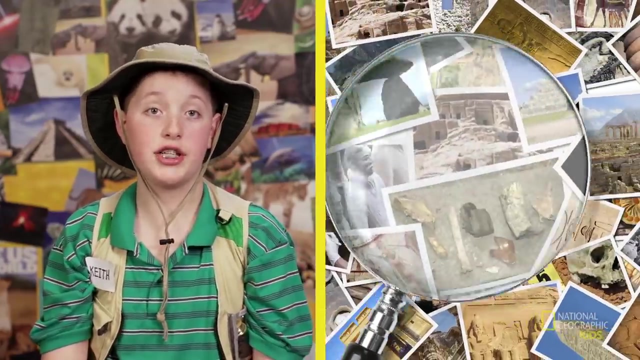 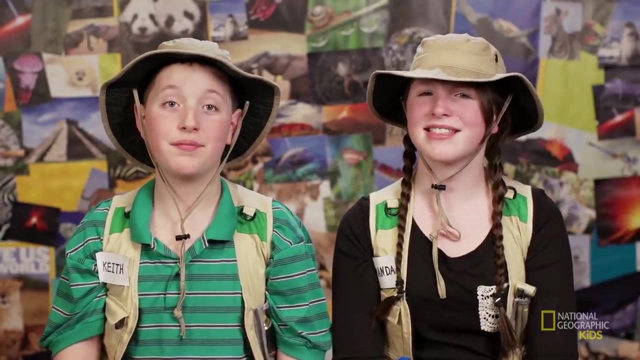 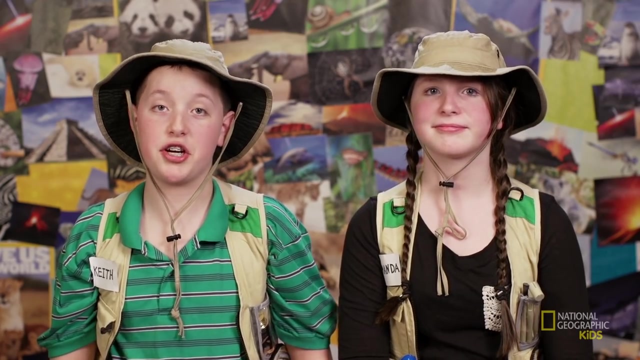 It's a great big world with so much to learn with National Geographic Kids. That can be anything, including buildings, artwork, tools, bones, weapons, even garbage. That might sound like digging for buried treasure, but the real treasure is in how the things we find tell a story about the way people used to live. 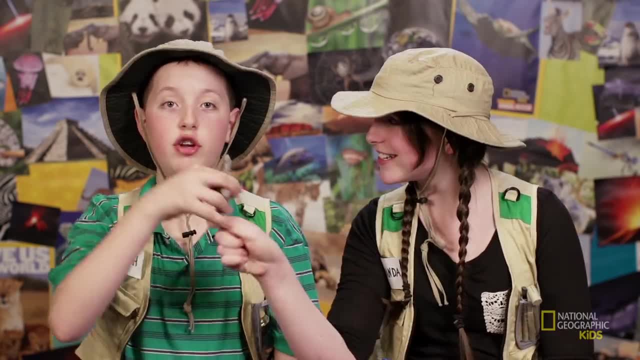 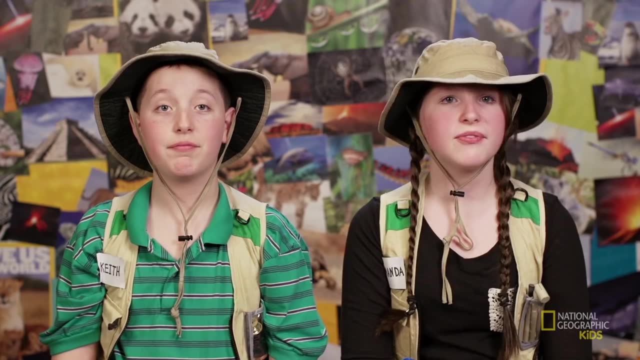 Does that include fossils and dinosaur bones? Nope, Even though archaeologists sometimes find fossils, what they really focus on are people and the things they leave behind. A lot of what we know about the people who lived before us was first discovered by archaeologists. 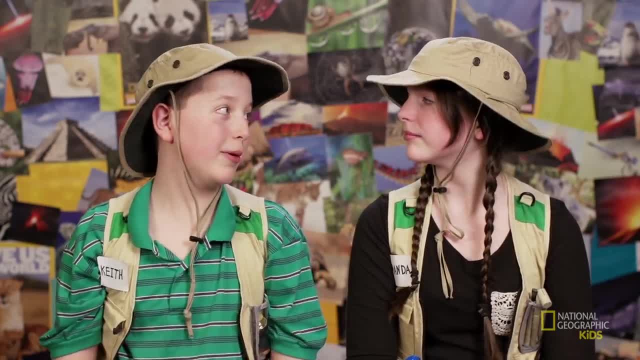 I think I'm ready to discover more about archaeology. Shall we dig in? 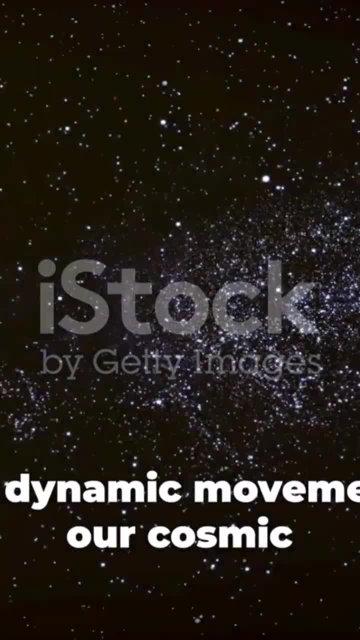 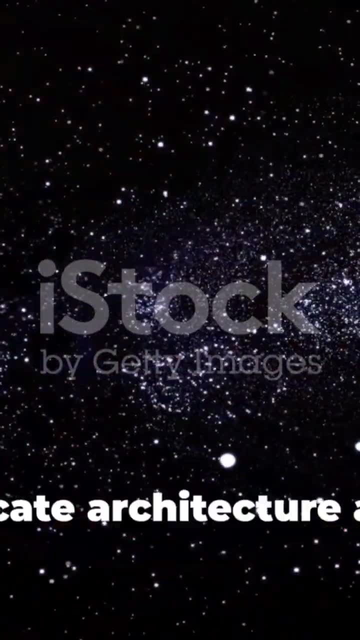 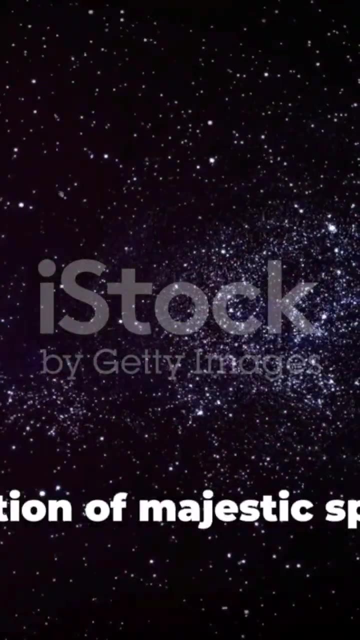 Venture with us on a captivating expedition through the grand spirals and dynamic movements that make up our cosmic dwelling, the Milky Way Galaxy. Discover the intricate architecture and rhythm of our galactic spiral arms, unveiling the breathtaking splendor and complexity of our celestial neighborhood, From the formation of majestic spiral arms to the gravitational dance.